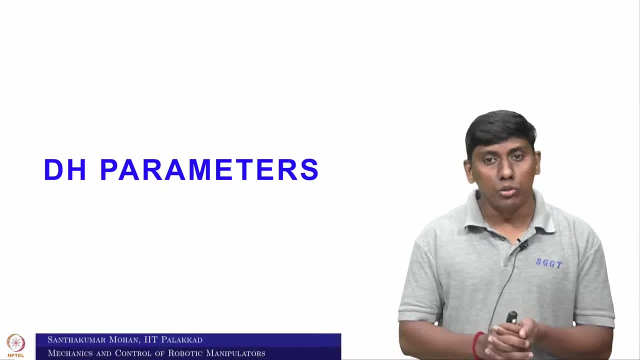 we call it is relative information of 2 consecutive joints, right? So in the sense we said that the relative information of 2 consecutive joint can be expressed in terms of one angle and you call one distance. So we will see like that how we can actually like pictorially. 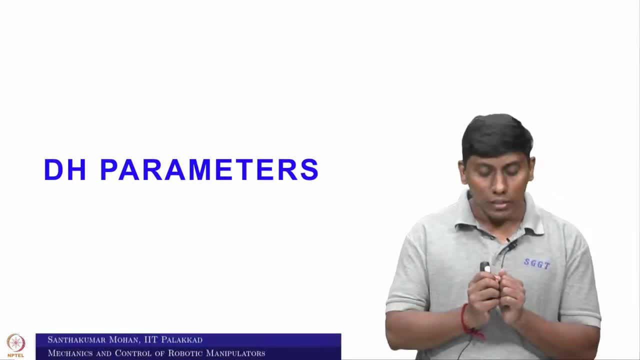 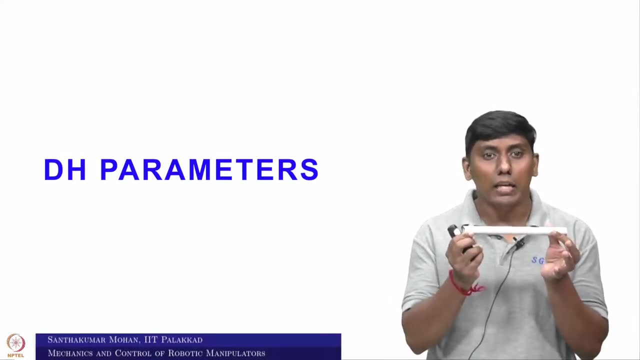 we can represent and, as well as physically, how we can feel it. So for that we are taking one link, you can see. So this is what we can call as a link now. So this is a random link, which is we call link k, or you can say link i-1. okay, So now you can see that this is. 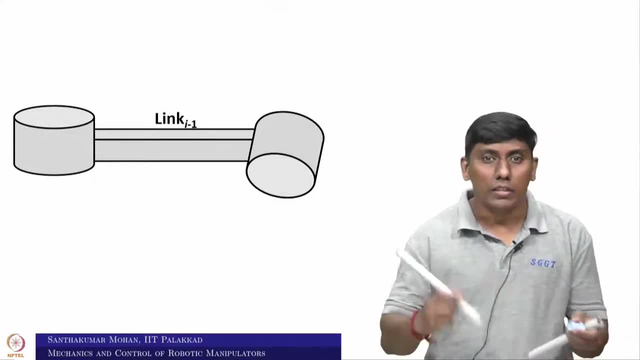 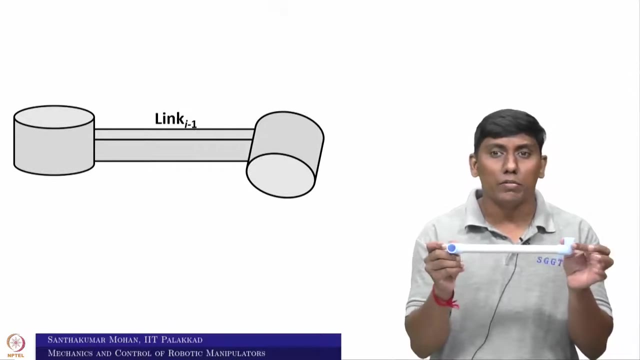 a random link. So this link would be having actually like set of things So you can actually like put it. you can see, I am actually like showing it. So this is what now become a link. So now this link is having something like arrangement, So very simple arrangement, which. 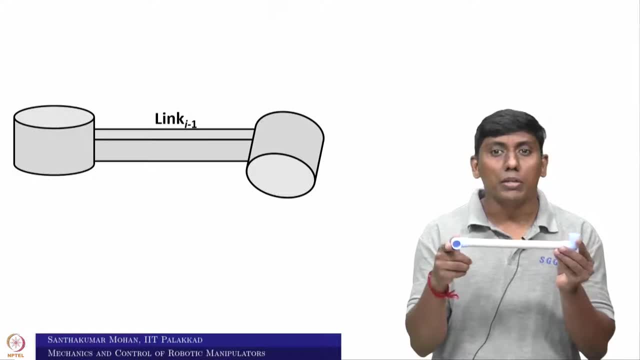 you can see, one elbow is actually like coming towards you, One elbow is actually like pointing upward. So now this link would be having what? so so many joints? So, as per Danowitz Attenberg what it says, any link supposed to be a binary link. So 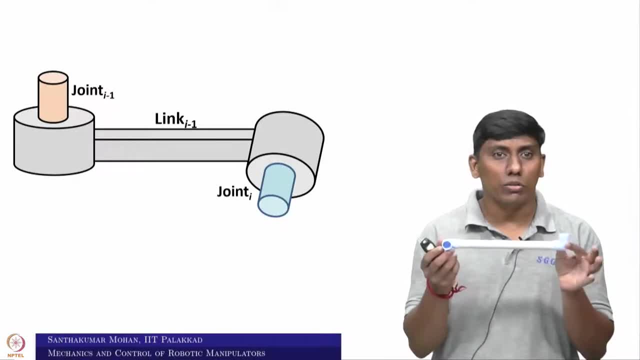 in that sense it would be having 2 joints. So what are the joints you can see? So these are the 2 joints. So these 2 joints, I am actually like pictorially represented there, that physically I am showing that this is one joint, okay, And this is another joint. you can actually 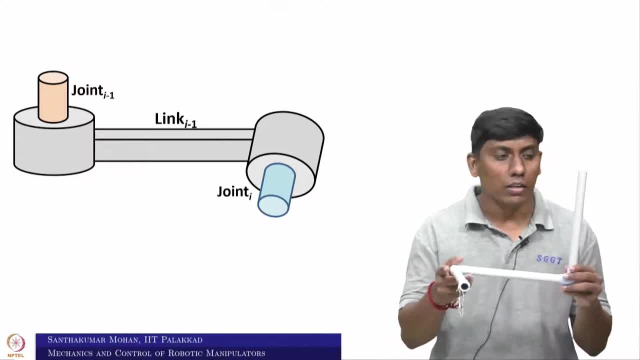 like see it. So now, if I connect this, you can see like one joint is actually like going upward, Another joint is actually like going inward, in the sense it is pointing inverse to you. So now this is link I – 1.. So this is a link. sorry, this is joint I – 1 and 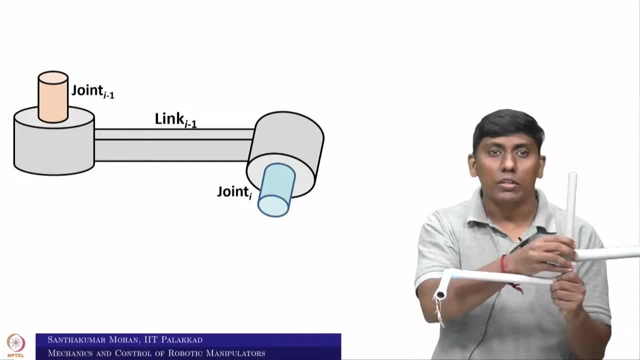 this is joint I. So this joint I – 1 would be having, you can say link I – 2 and link I – 1.. So this, this link, what you call this link K, link I – 1 on the joint I, it would. 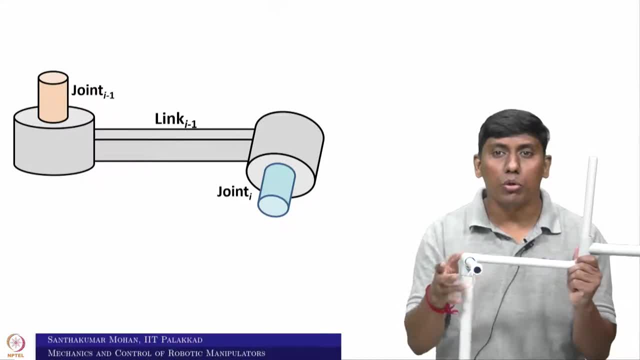 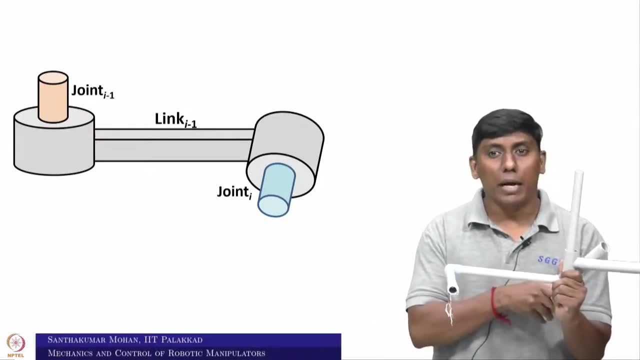 be connecting. So one more link, So, which is actually like what you call. So this is link I, So this is link I and this is link I – 1 and this is link I – 2.. So now, in that sense, if you take a random link, you can see this I – 1.. So what you can. 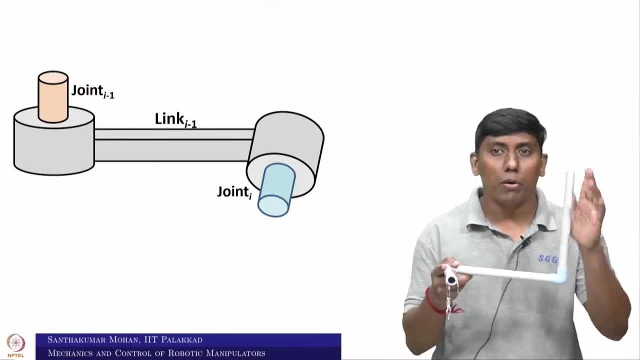 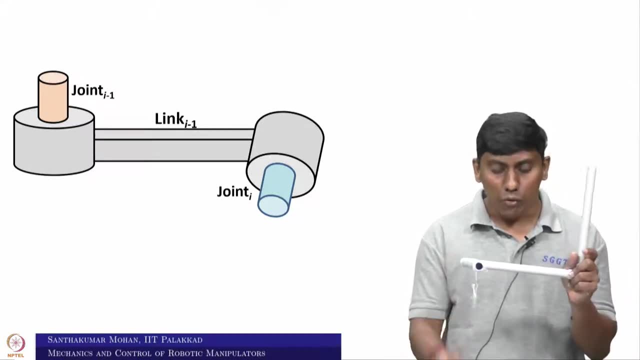 see it would be having 2 joint axis. So one is actually like pointing out, you can say up, So that is what we call joint I – 1.. So the other one is actually like joint I. So now, as per our you can say Danowitz Attenberg approach, what we can see these 2 joints are 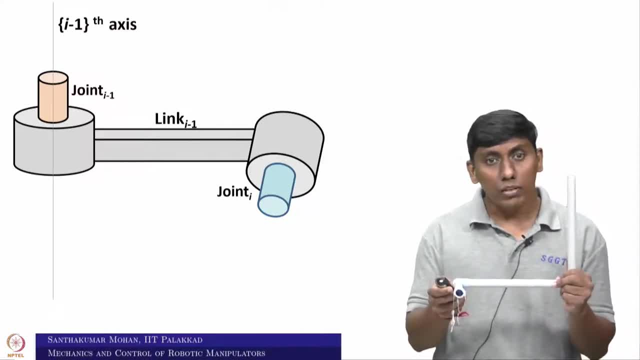 supposed to be fixed. So this is the joint I – 1.. So this is the joint I – 1.. So this is the joint I fixed in. you can say axis, So this is actually like can be rotary or actually like a translation joint, But what we can actually like see that these 2 axis. 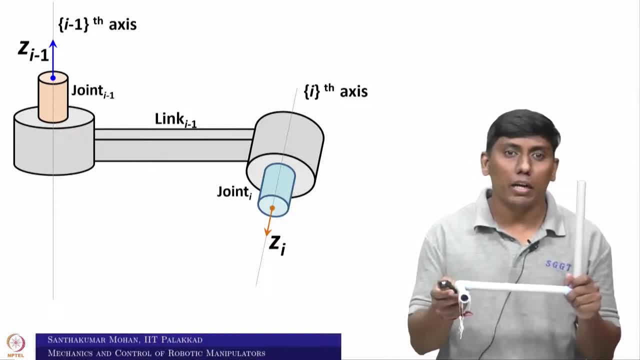 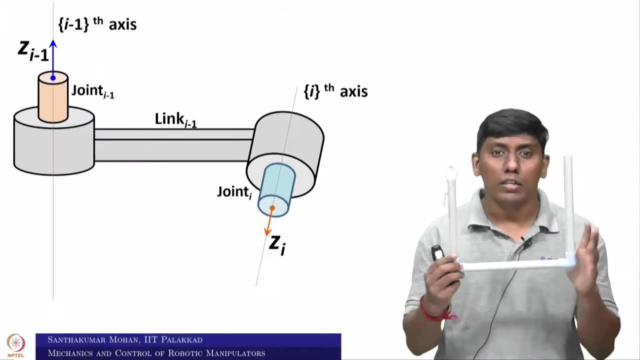 supposed to be fixed with Z. So in the sense Z I – 1 and Z I would come. So now what it is giving. So this link I – 1 is giving a relative information of this joint I okay this joint I and joint I – 1.. 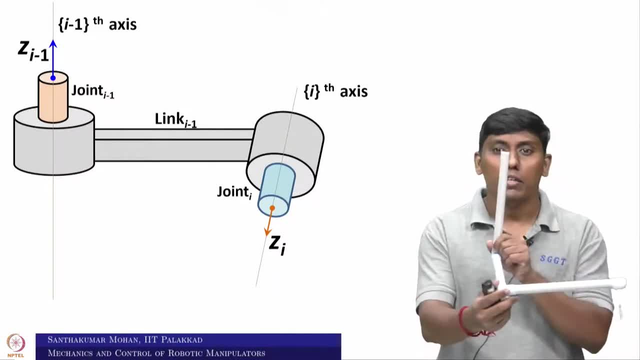 So now you can see that these 2 are actually like how you can look at it in the front view You can see these 2 are actually like angle apart, and in the front view you can see it is distance apart, right? So first we will actually like attempt: what is the joint angle? 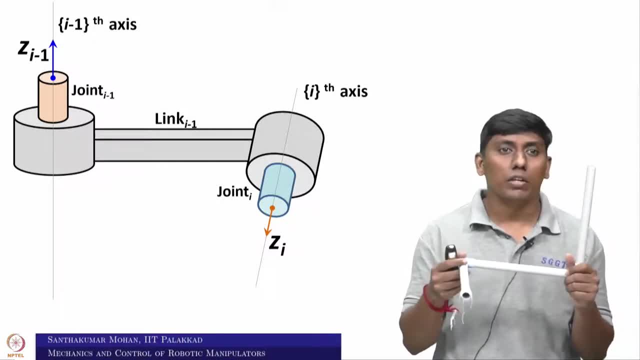 apart, or you can say the angle apart. So these 2 joints. So for that, what one supposed to do? we have to draw a common normal between these 2, what you call joint axis. So I am doing that. So now what you would did. So we drawn a common normal between these 2 axis. 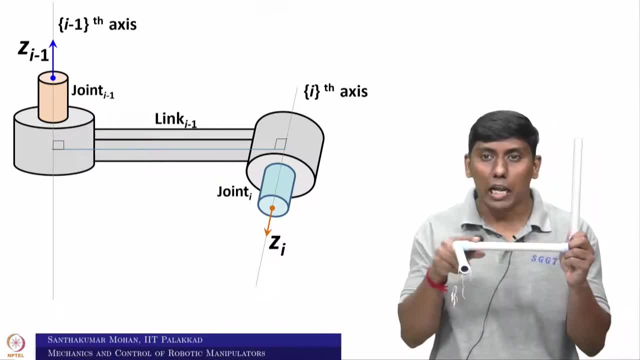 which is actually like coming on this line right. So now, in this line, if you look at it, what you can feel it. So this is actually like a travelling line and, as well as you can see, that with respect to that, you can rotate right, either this or this you can rotate. 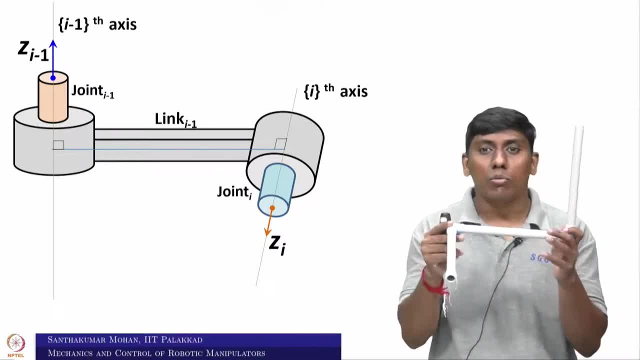 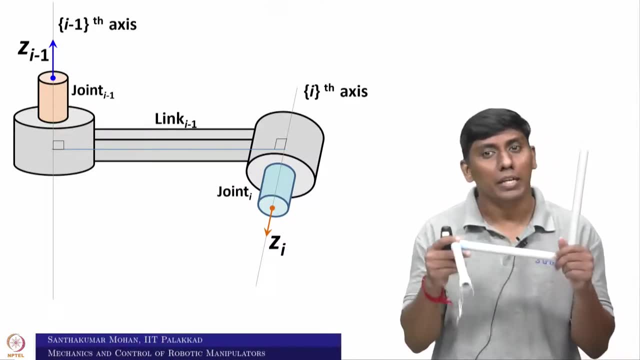 So now we are actually like taking this line, some axis, So what axis? as per the Dynavit-Atenberg, So on the link, so you will take link parameter would be represented with respect to x axis. So in that sense this you can say common, normal, what you have drawn. So on that you can actually 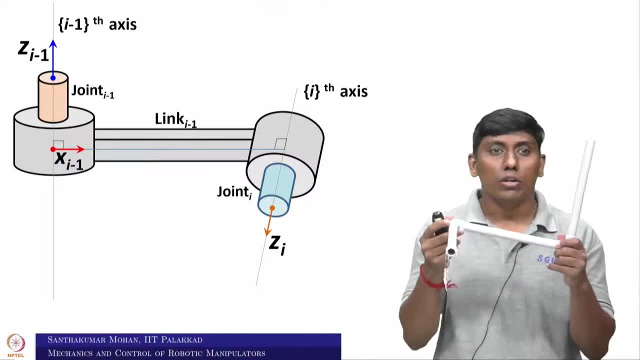 like fix the x I – 1 axis. So now what you can see, this is what your joint I – 1 and this is your joint I, So the common normal you have drawn, and this is the point, what you call the frame point. 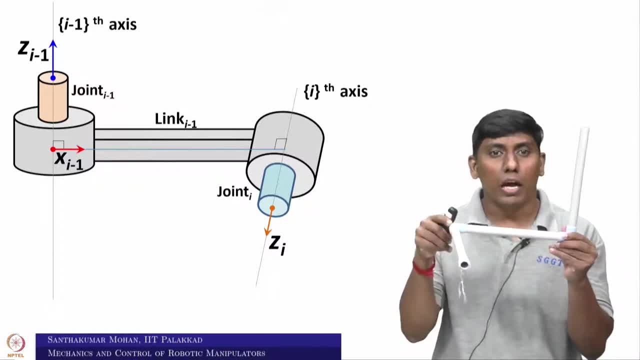 So now the point, which is actually like coming towards your I, So that is what you call x I – 1.. Now, with respect to this, what you can do, you can actually like rotate this right So you can look at it. So this is actually like your x I – 1.. So now you are actually 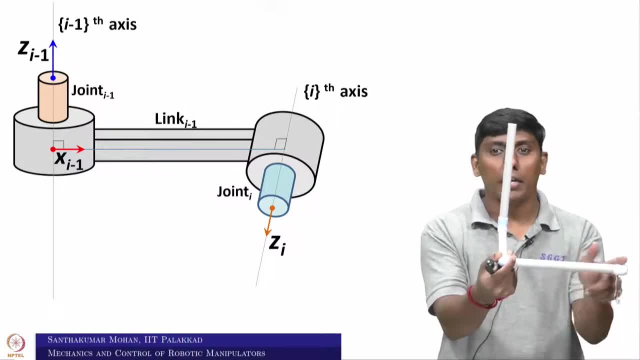 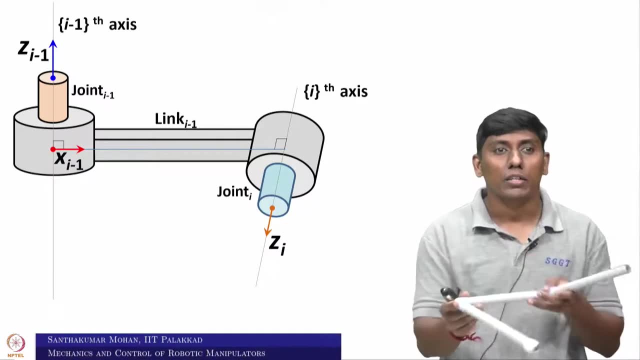 like rotating. So now, what one can see, this is joint I and this is the joint I – 1.. So, in the sense, what one can see? you can rotate this much angle and make it parallel. So that is what we are actually like doing it. So what first we are doing it. So this is what you have. 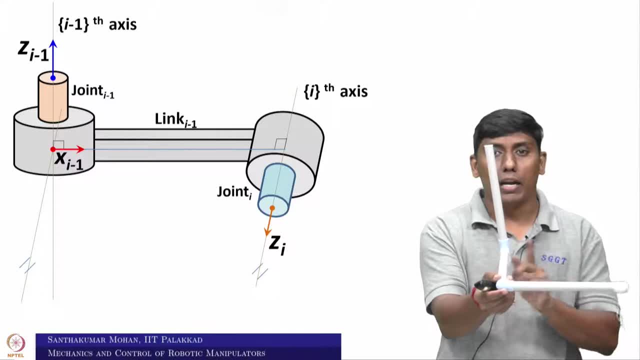 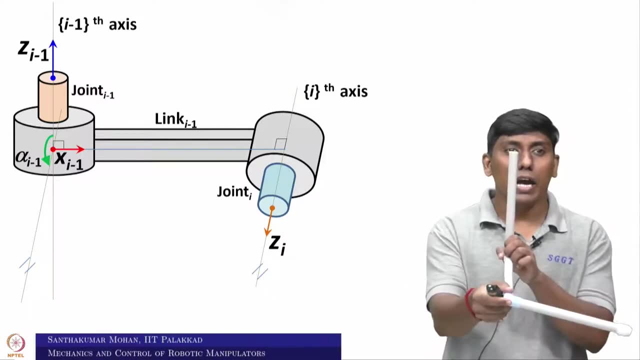 joint I – 1 and this is joint I. So I draw a parallel line from this point. So now I have drawn, then I will rotate right. So that is what I did. So how much angle I rotated with respect to this. So this is actually like with respect. 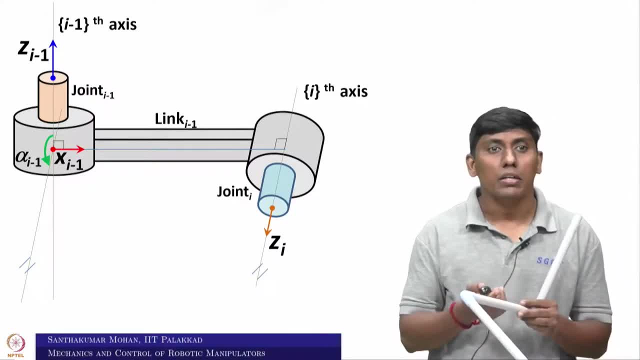 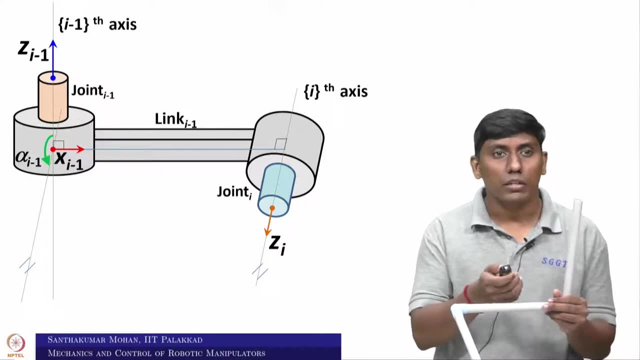 to this axis. neon죠, you have rotated, so alpha i – 1, so the alpha i – 1 positive direction also. you know right, so that what we have actually like done here, okay, So now this is giving one angle call. so these are the two. you can say joints. this is twisted. 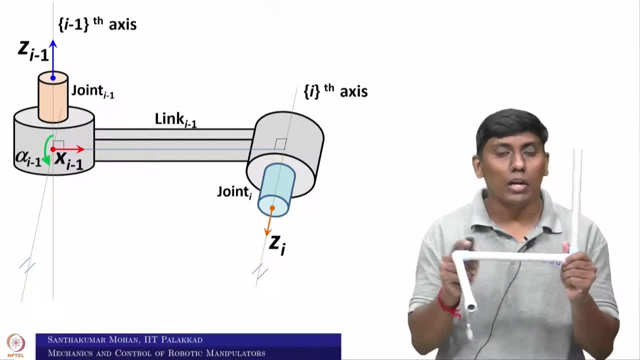 so that is why it is called link twist. so this is with respect to link. so these two joints are twisted, so that is why it is called link twist. so this angle represented as alpha i – 1, this is about xi – 1 angle between zi – 1 to zi, what you call link twist angle. 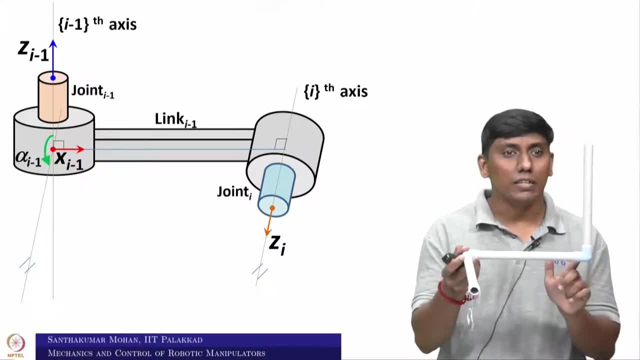 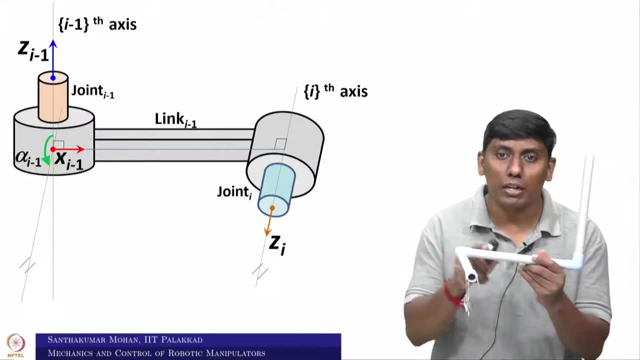 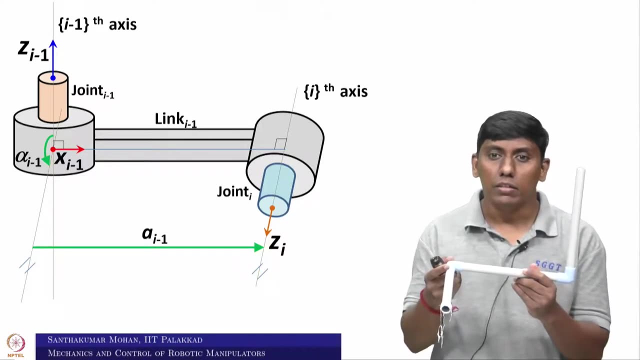 okay. So now, what else is remaining? you can see, like the distance between this point to this point. so there is actually like a travel across, right? so in the sense, what you can see, so you can actually like go across and then see it. So now this is what, the distance, which is what you call ai. okay, if you are actually 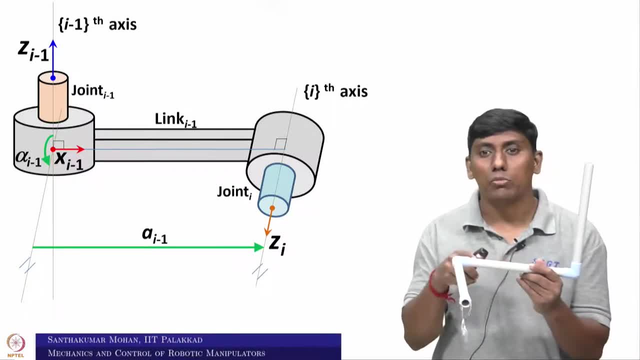 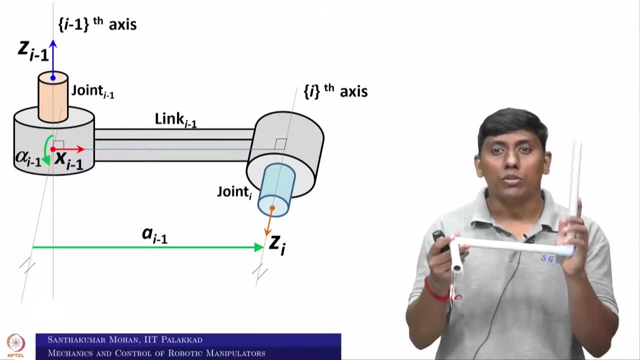 like representing with respect to i – 1.. So this is ai – 1, so in the sense, the frame distance, in the sense you have zi – 1 and zi, so the angle between these two, what you call alpha i – 1, the distance between these. 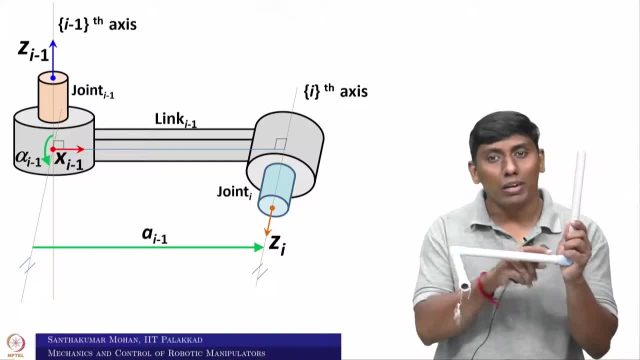 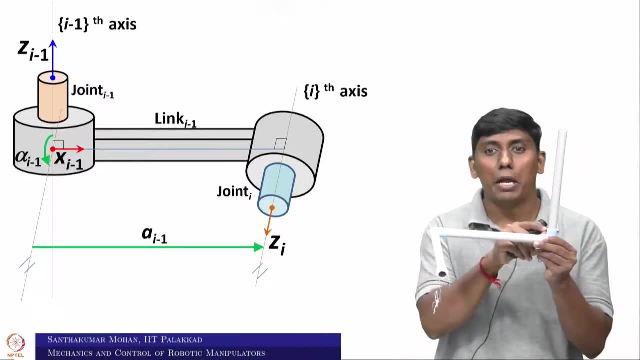 two about or along xi – 1, what you call link length. okay, So why it is called link length? because this length is actually like 0. what you can see, these two frames are actually like in the same point. so now there is a physical length. 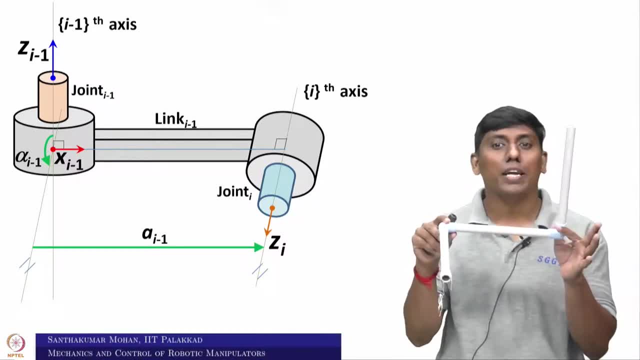 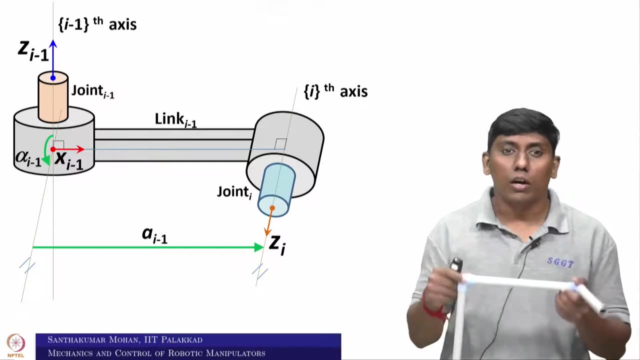 it is actually like distance apart. So that is why we said the physical length cannot be negative. So we have to take xi – 1 always on a progressing side, okay? So that is what we written in the previous lecture. So ai – 1 should be always positive or 0, okay. 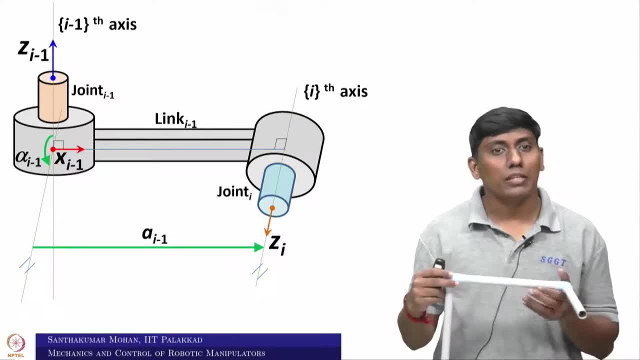 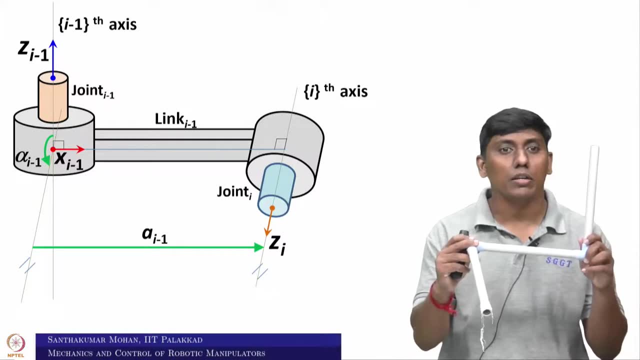 Now you got these two what you call link parameter. So one is actually like angle between zi – 1 and zi about xi – 1. that is what you call link twist. So it is nothing but a twisting of these two joints about this link. 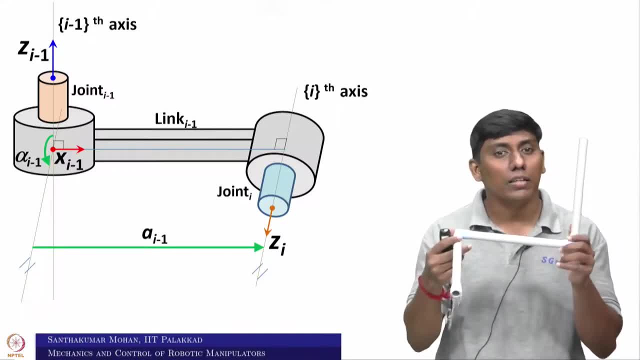 So that is why it is called link twist. So the other one is actually like these two axis, how much distance apart along xi – 1, that is what you call physical length, which is nothing but link length. Now, the same way, we will actually like see what you call the joint parameters. 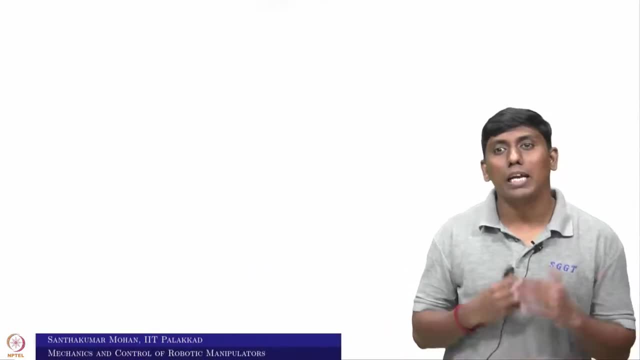 So what are the joint parameter? So joint parameter will talk about the relative information between two links. So now we will take a random joint. So for that I am taking a random joint. So now this is actually like we call, actually like a joint. 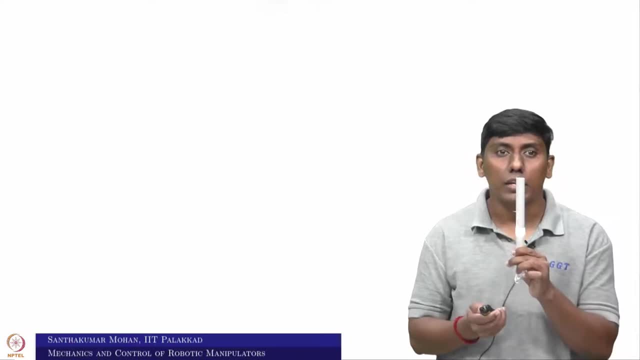 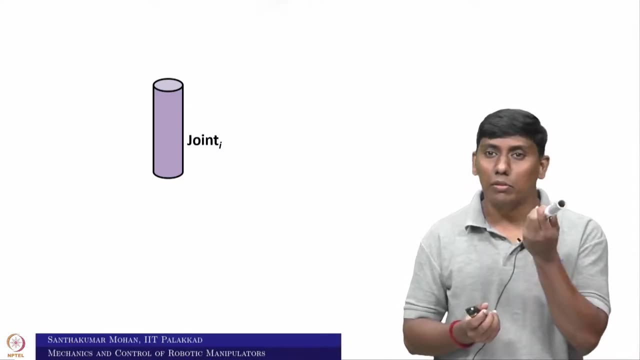 Okay, So this joint is actually like joint type, okay. So now I have actually like taken the same thing. in the picture You can see. this is what the joint, which is nothing but a PVC pipe. There you can see a cylinder right. So now this joint is connecting what? 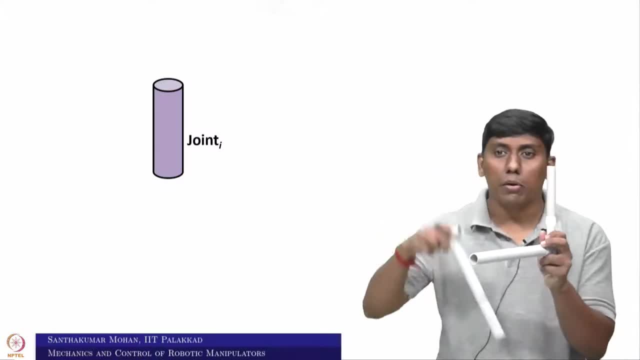 So there are two bodies, right, So one body and another body, right, So now what you can actually like look at it. So this joint will give a relative information between these two joints. So how much distance apart, okay, and how much actually, like angle apart? 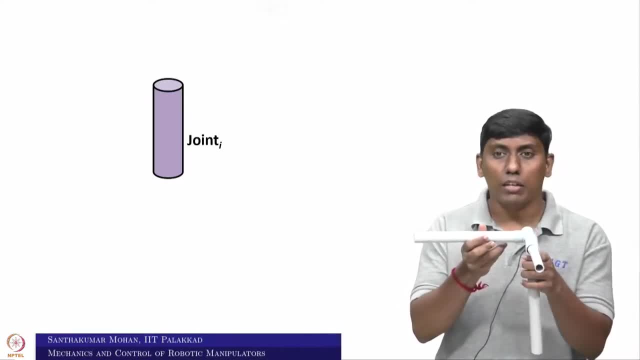 So if you look at in the front view- or you can say you talk it, this is as a top view- You can see that these two links are actually like angle apart. So if you look at it in the front view, you can see these two links are actually like: 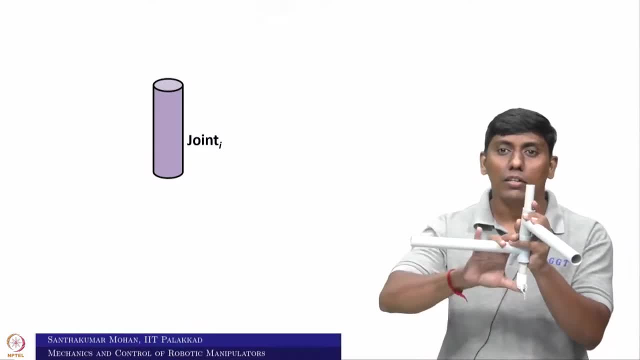 distance apart. right, So you can actually like look at it, right? So this is what the distance and this is what the angle. right, So now these two, you can say parameter, that you call the joint angle and the joint length, or you can say we call 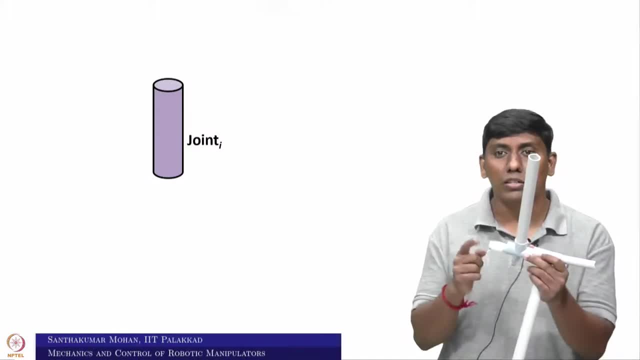 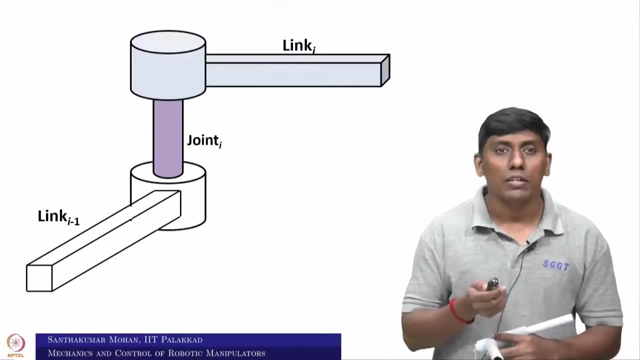 That is joint distance. Okay, joints can be expressed on what? so this joint axis, right? So, whatever this, this is what going to represent. So that is what we are trying to explain here. You can see that these are the two links we have connected. 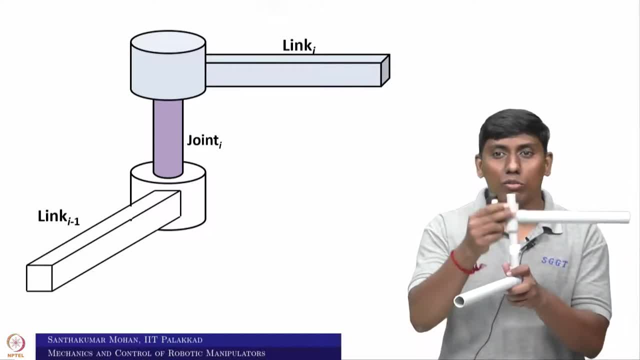 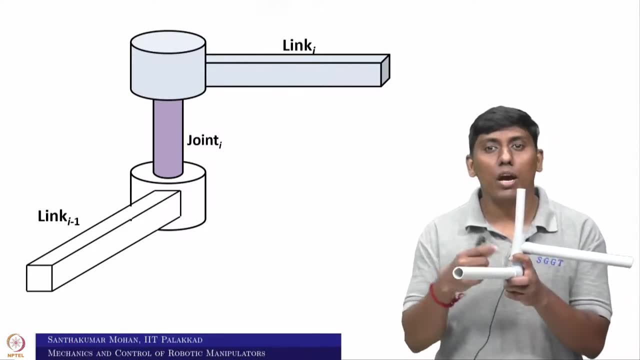 Now these two links are actually free about this joint. It can actually like translate or it can actually like rotate about this. So now you can see like these two links supposed to have some, you can say, phenomena. So first, what we will fix, We will fix the joint axis. 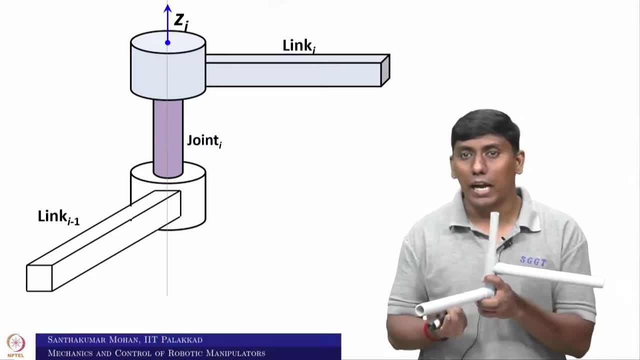 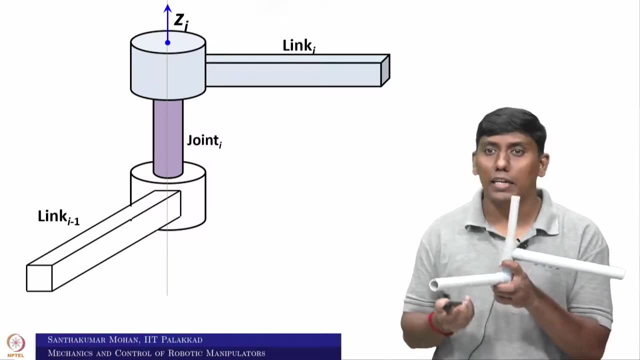 So, as per the Danube-Tartan bug, this joint axis is actually like Zi. So now Zi is fixed. So now the link would be having what Link parameters? The link would be having Xi and Xi-1, right. So that is what we fixed here. 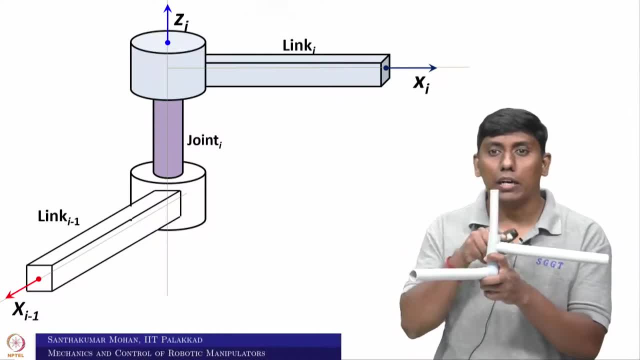 So now you can see that this Xi, which is actually like going here, and Xi-1 is going here. So now if you look at in the- you can say top view, So you can see like these two are having angle apart. So that is what you can actually look at it in the figure. 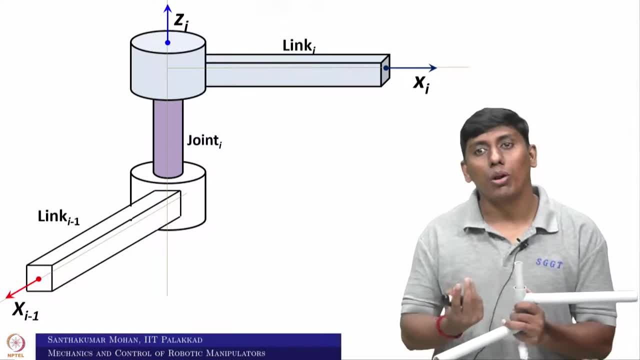 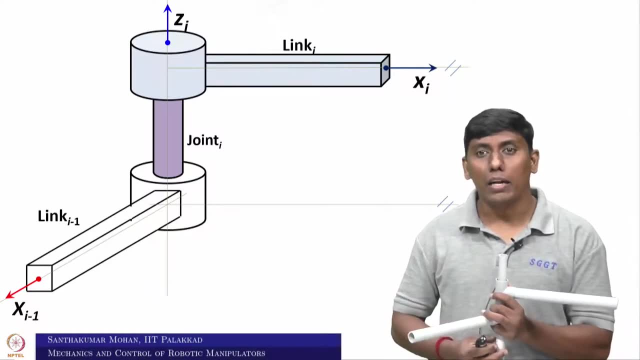 The angle between Xi and Xi-1.. Okay, Okay, So that is what we are trying to do. So for that, we are actually like making a Xi parallel line at the you can say link i-1, and you have actually like drawn that. 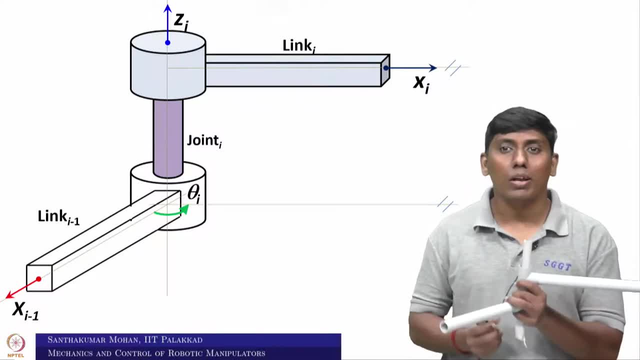 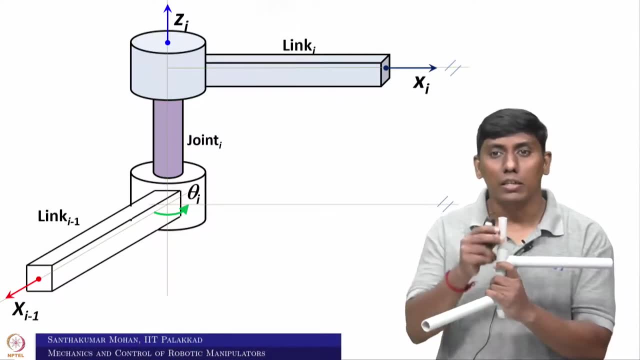 So now what you can see, the angle between these two, what you call joint angle. So this is actually, like you can say, referred with respect to the particular, you can say joint axis. So now, what is joint angle? So you can assume that these two are actually like parallel. 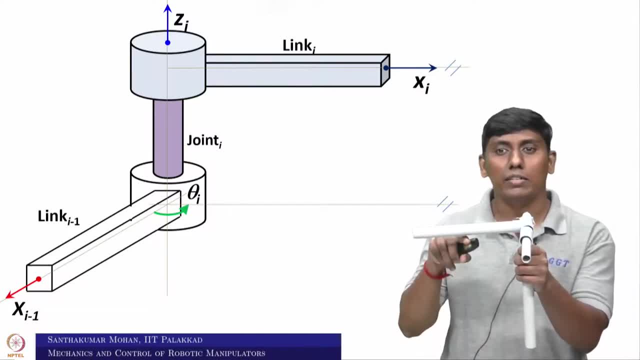 So now it is rotated. What would be this? So now, theta i is there, This is what your joint axis. So now you can see: like the theta i is there, So now what is the joint distance? The distance between these two, you can say axis. 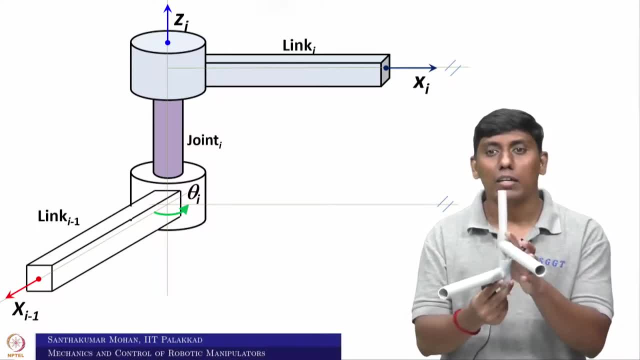 Now what it look like. It is actually like. look like it is a half planer, right. How much it is actually like offset between one plane to another plane. So that is why it is commonly called offset distance. What you can see, So you can see like: this is link i-1 and this is link i. 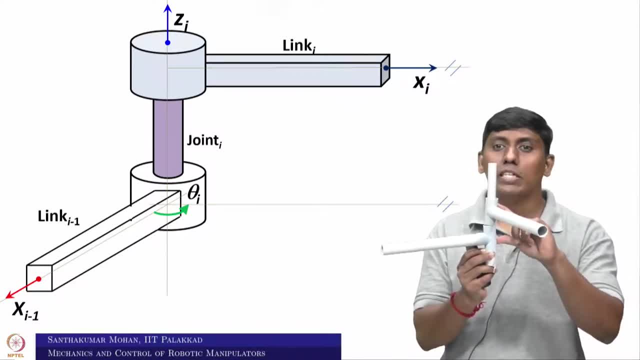 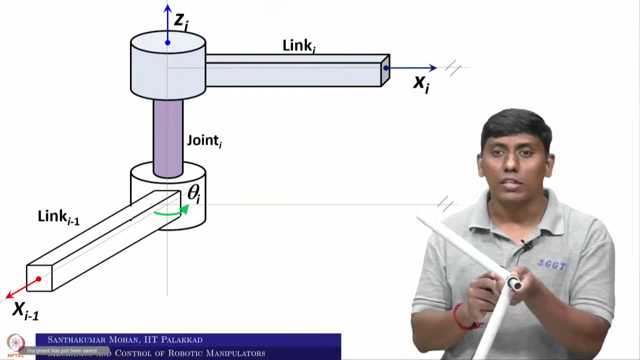 So how much it is actually like planer offset This much distance. So which axis you are referring? Xi, right? So this is what the you call joint distance or offset distance, So the angle you can see in the top view and the distance you can see what you call from. 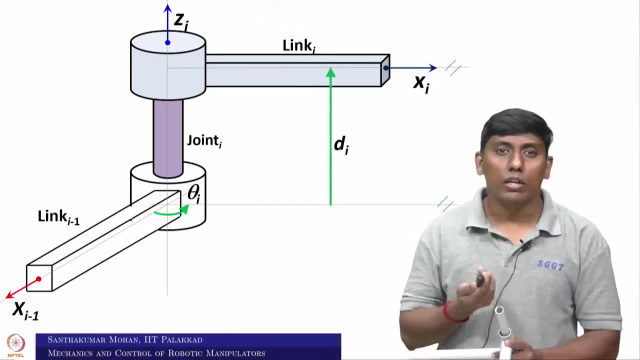 the front view. So now, this is what the joint distance, So that is what we have actually like written. I hope now it is actually clear. So what is Dynavit Attenberg parameter? So where is it? Here you can take a random link. 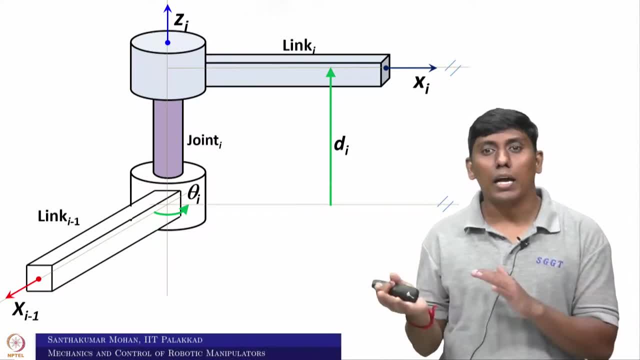 So that link would be having two joint axis. So these two joint axis information which is giving that is what you call link parameter. So this link parameter is a constant, or you call it is a geometric parameter, because once you fix the link, so that link cannot be changed. 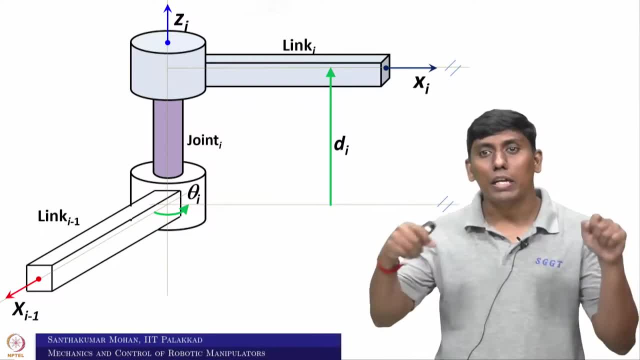 So in the sense you take actually like one random link, that link configuration will not change time to time, Whereas you can take the joint. So the joint would be actually like connecting two consecutive links. So now the relative information between two links would be given with the joint. 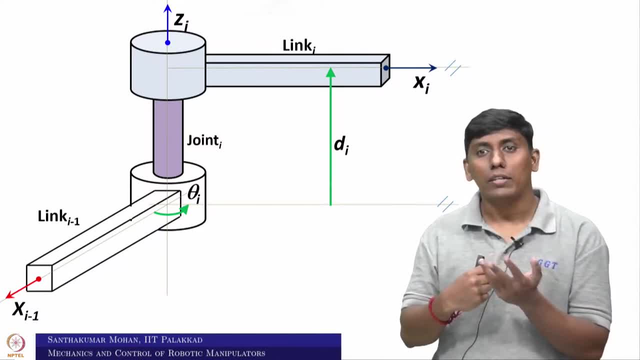 So that is what you call joint distance and joint angle. okay, So that actually, like referred to joint axis, which is Zi, whereas the link parameter is geometrical parameter that referred with respect to you call Xi – 1.. So now you got the clarity between what is link twist, what is link length, why link? 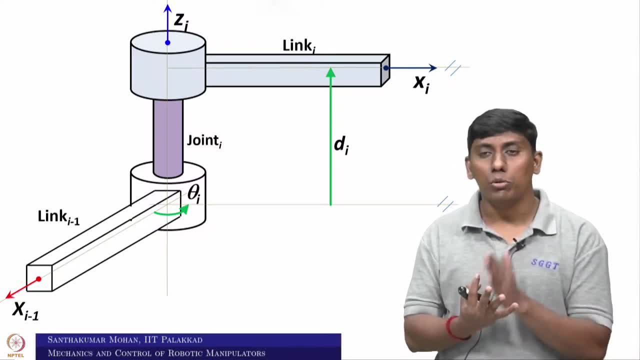 length is actually like, should not be. you can say negative. You got the physical field. Similarly, what is joint angle and what is joint distance? why joint distance is called, as you can say, offset distance? These all actually like. I hope you are clear. 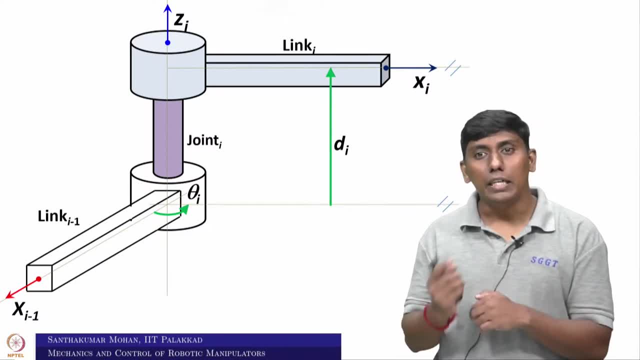 So whenever you call theta, so theta referred to I, D referred to I, So in the sense you are referring to the joint axis which is Zi. So in the sense theta, I and Di would be corresponding to ith frame, whereas you can say the link.